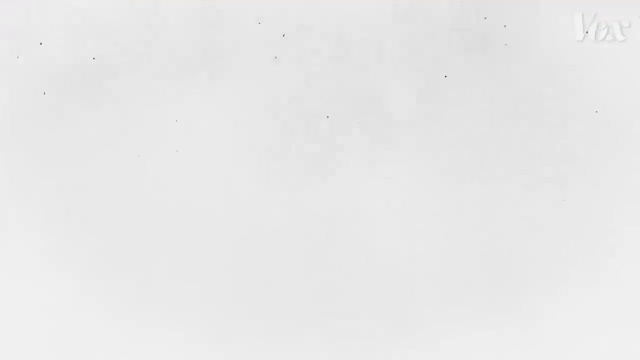 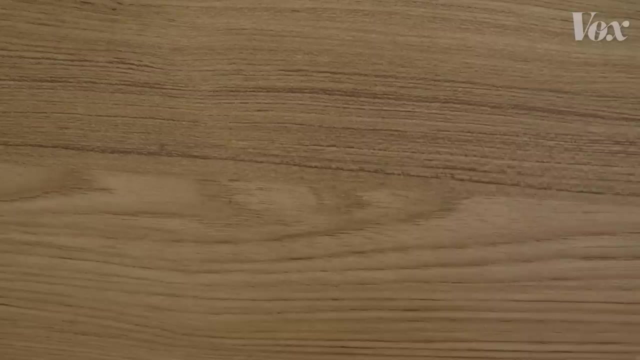 Here's how the current scoring system works. Skaters perform two routines- the short program and the free skate- and they receive two sets of scores for each. The technical element score evaluates the difficulty and execution of a skater's jumps, spins and footwork. 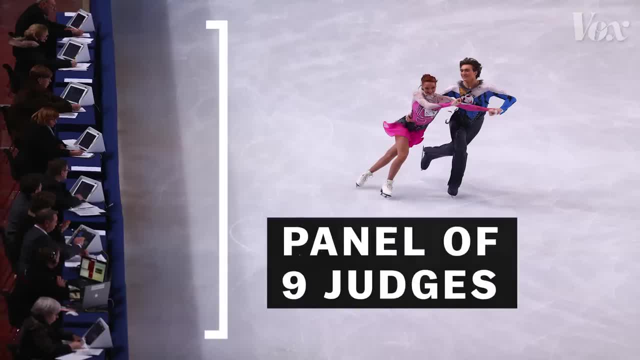 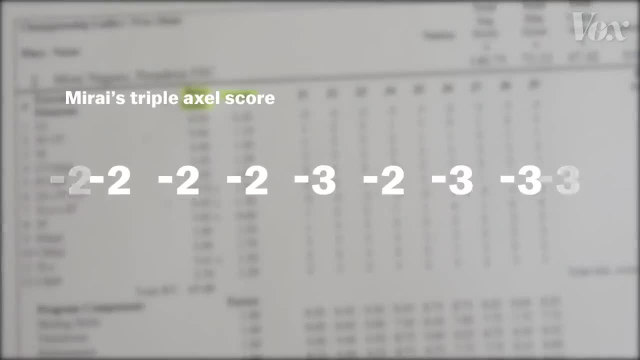 Each element has a base value and a panel of nine judges provides great evaluation. The score is then divided into three categories of execution scores, which range from plus three to negative three. The highest and the lowest scores of the judges are ignored, and the average of the remaining seven scores is added to the base value. 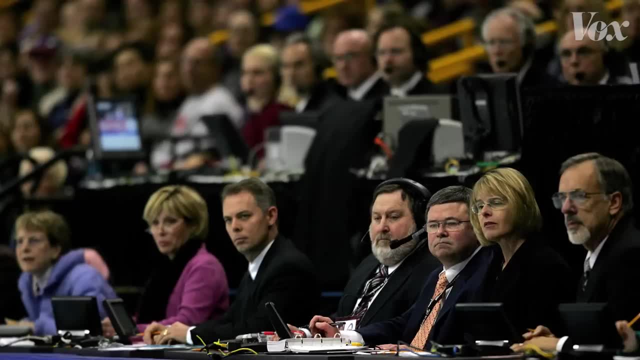 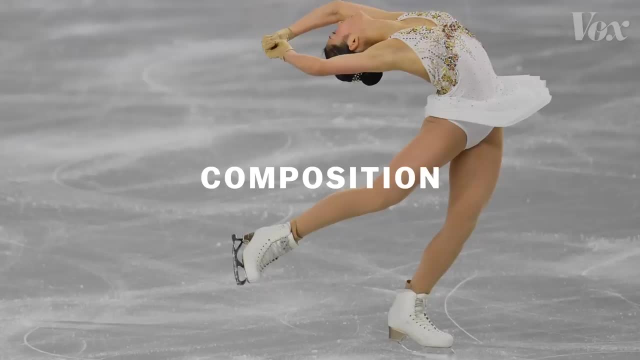 The program component score judges a skater's presentation or artistry Judges. award points from 0.25 to 10 on the main program components, including skating skills, transitions, performance, composition and interpretation of the music. All together, the combined total score of the short 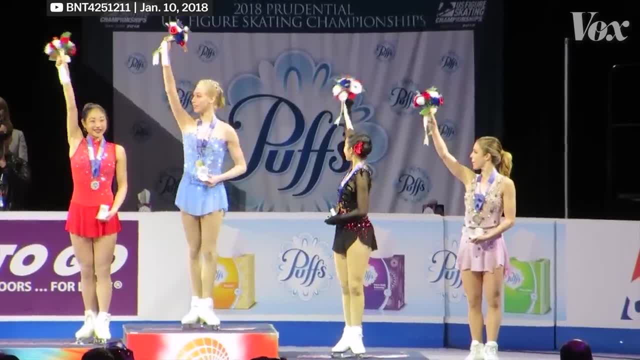 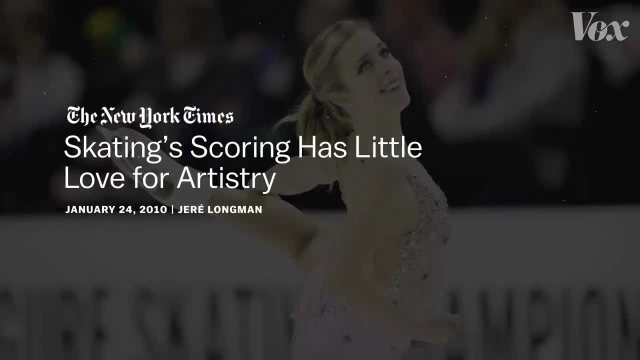 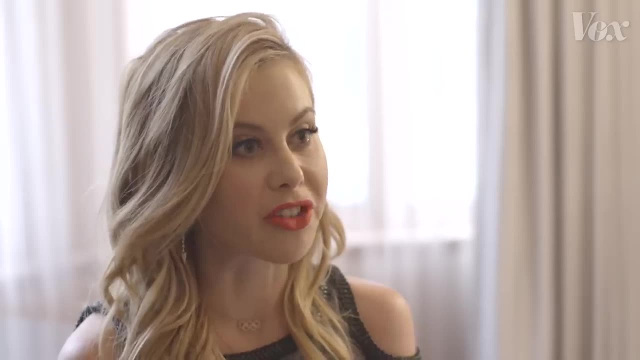 and free skate determine the final standings. The goal of this new system is to make every element accountable for, And while it has, the system has also had a huge effect on the sport and the skaters themselves. You're seeing a lot more skaters now try all these quads and the program becomes messy because 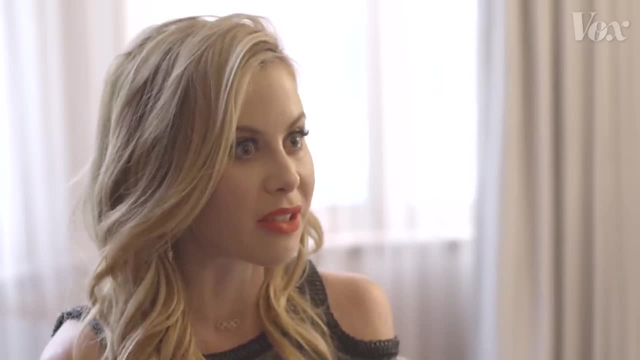 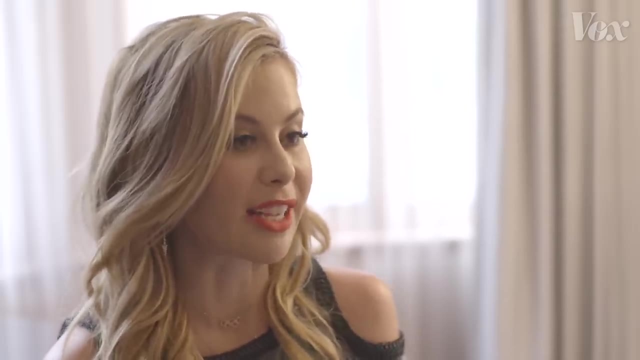 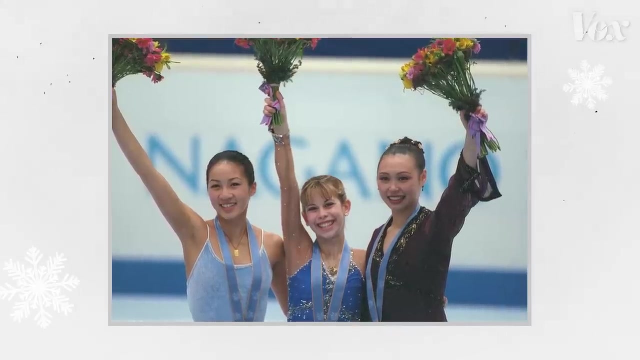 maybe they're not so consistent on it, but they're hoping that, because it's a good base value, that they can up their technical score and then their artistic score starts to lag behind. That's Tara Lipinski. In 1998, she became the youngest person to win an Olympic gold for the ladies single event. 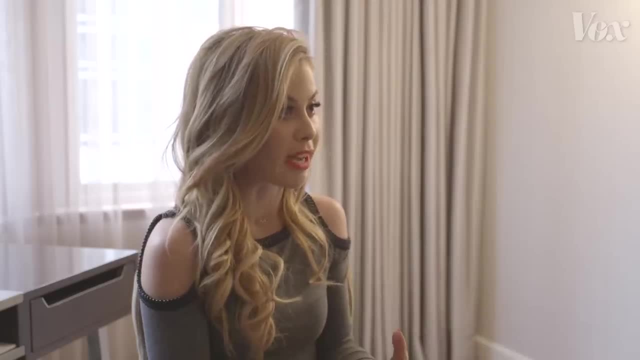 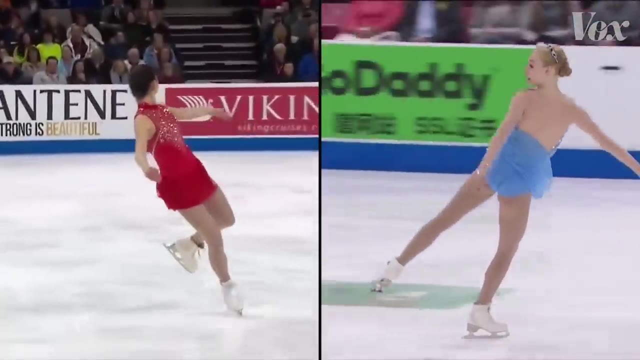 Some of the skaters are losing the artistry because they're trying to cram in everything and they're not prepared for it. yet The system rewards risk and difficulty. Merely attempting a difficult jump can earn a higher score than perfecting a slightly simpler jump. 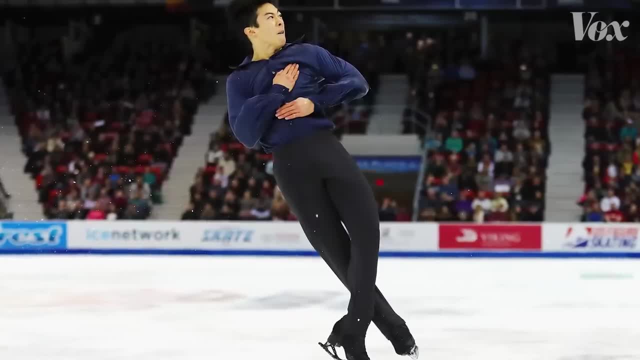 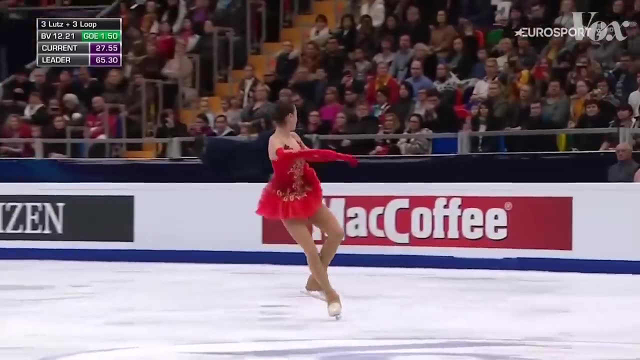 Skaters can increase their grade of execution scores and earn bonus points for things like placing jumps into the second half of the program. This is an amazingly challenging program. Every single jump pass is in the second half, or completing a jump with your hands in the air. 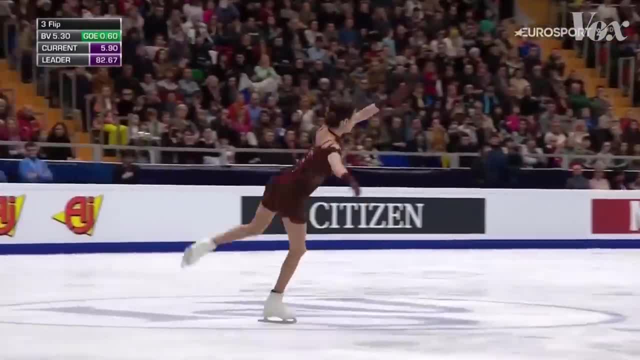 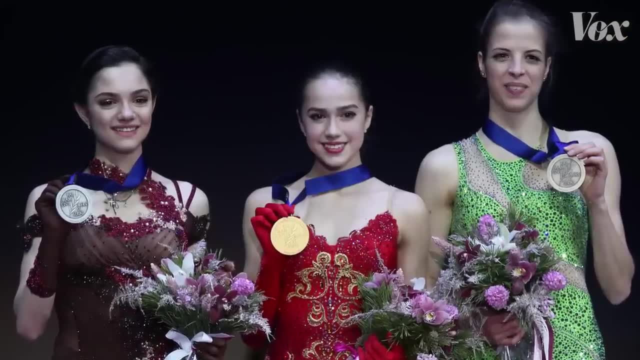 But arguably it seemingly gives less incentive for skaters to simplify their routines and perform elements cleanly. If they do, they won't be able to win. At the 2017 Four Continents Championship in Gangneung, South Korea, Mariah's fellow Olympic team won the gold for the ladies single event. 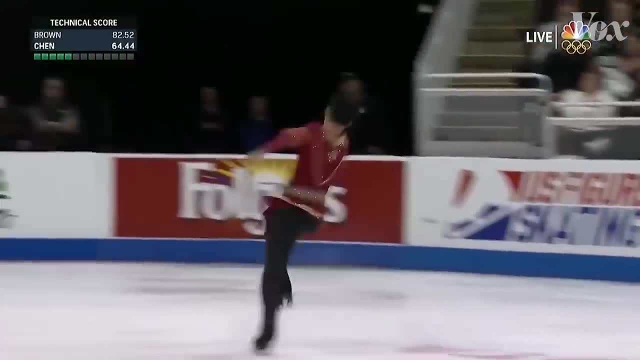 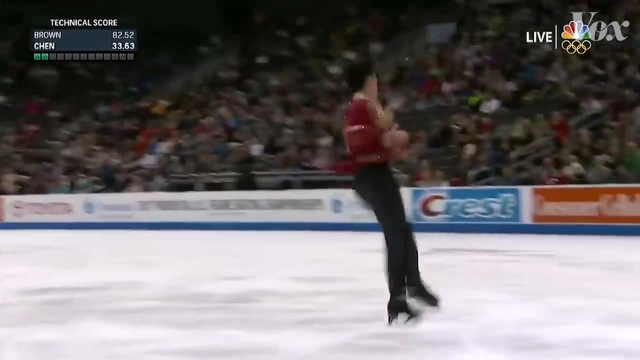 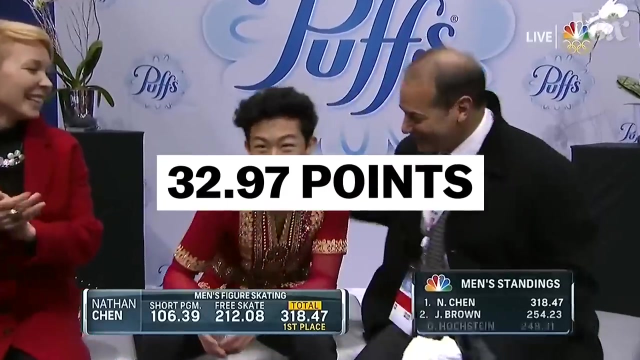 Her fellow Olympic teammate, Nathan Chan, won gold and became the first and only skater to complete five different types of quadruple jumps in competition. That's five, the first time ever. Based on the difficulty of his elements, Nathan's technical score was 32.97 points higher than Jason Brown, who had no quads in his routine. 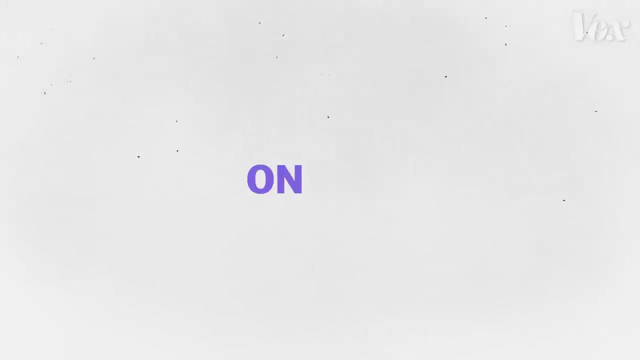 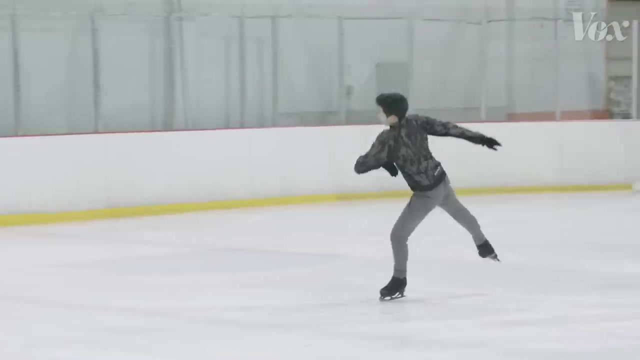 Unlike the program component score, there is no point limitation on the technical element score, So he can keep up with his natural and high-level skaters and improve his performance as he would have done without any technical elements. But artistry is still important, as it can be the difference between two skaters competing. 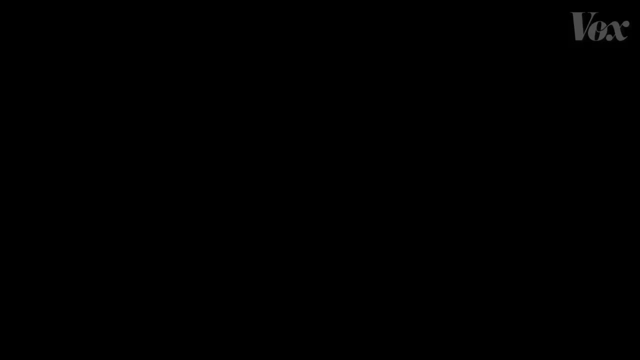 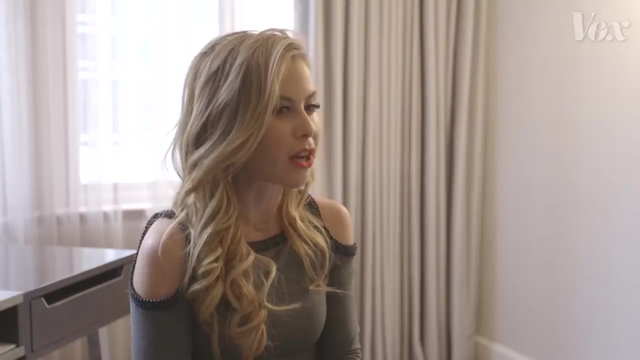 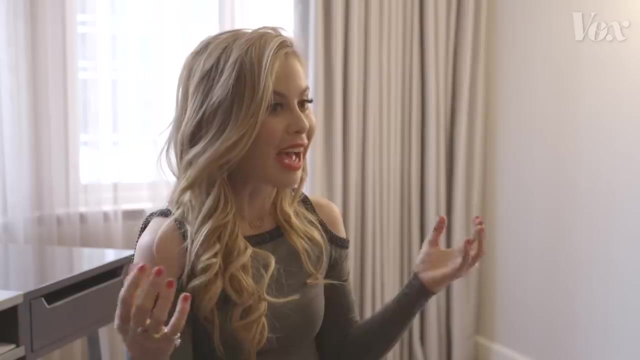 with similar technical elements. Pushing the difficulty envelope is not an inherently bad thing, As it helps the sport to evolve, But I also think at the same time we have to figure out a way to make these skaters have a clean skate. Because, at the end of the day, when you strip the drama and the politics of the sport, things you've experienced have been useless, But there are times when you can still get a great ski jump to improve it. Because, at the end of the day, when you strip the drama and the politics of the sport, 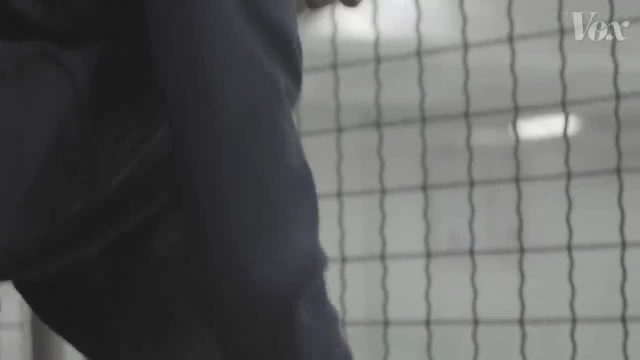 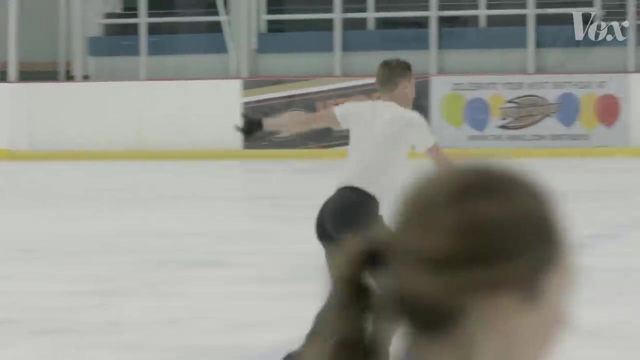 things you've experienced in your lifetime. things you've experienced in your lifetime At the end of the day, when you strip the drama and the politics of the sport, skaters, like all athletes, dedicate their lives training and working towards this one specific goal. 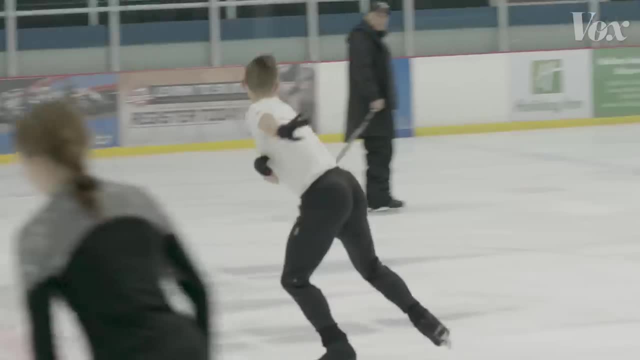 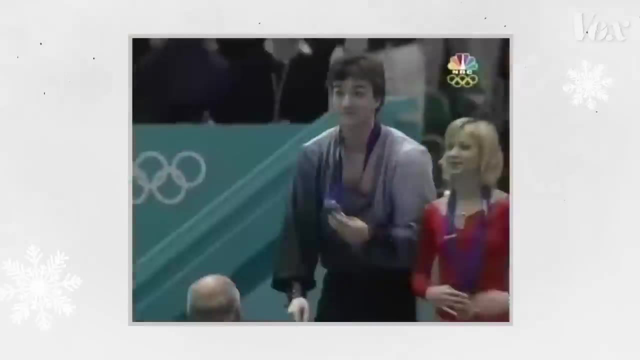 And they just want to be able to skate knowing they've been judged fairly. It's why we have the new system in the first place. When it was revealed that a French judge fixed the results of the 2002 Olympic pairs event so that the Russians would win, the new system was created as a step towards accountability. 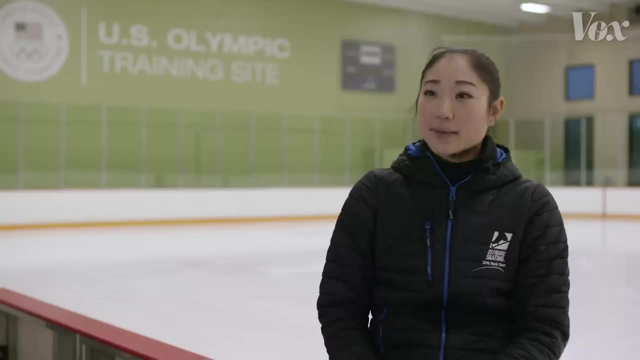 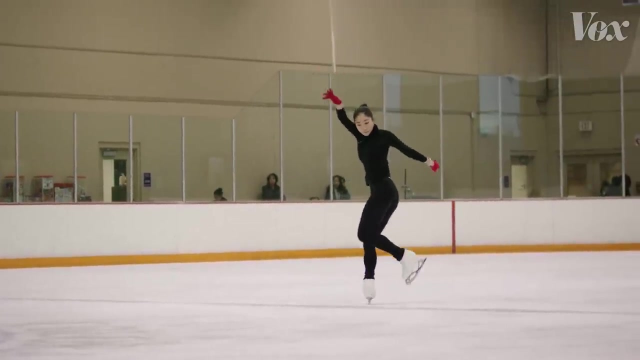 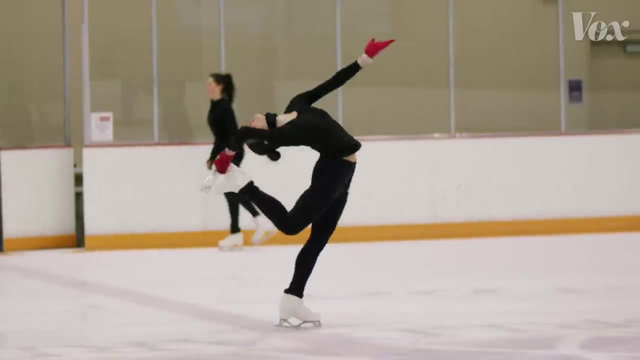 and decreasing subjectivity. Figure skating has always been a subjective sport and it's not like racing or basketball or hockey, where it's easy to see. But you know, performing is something I really love and I love skating, and so I try to follow the rules to the best of my ability and to garner as many points as I can. 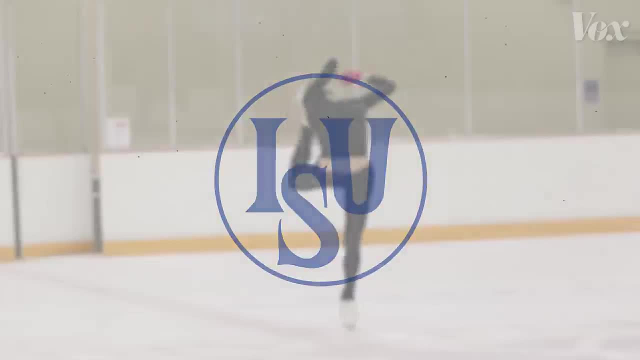 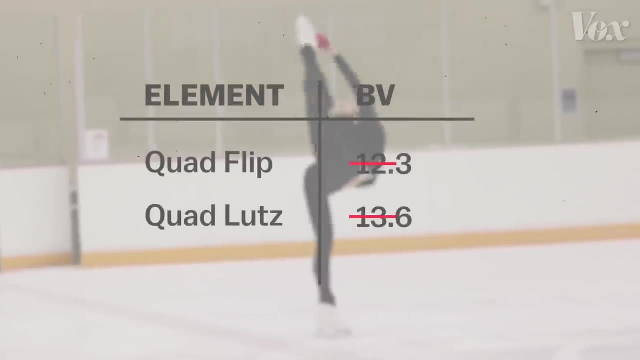 The International Skating Union, which governs the sport, says it wants to close the gap between the artistic and technical aspects of the sport. There are proposals to reduce the base value of quad jumps or have three different medals: one for technical, one for artistic and one for all-around.